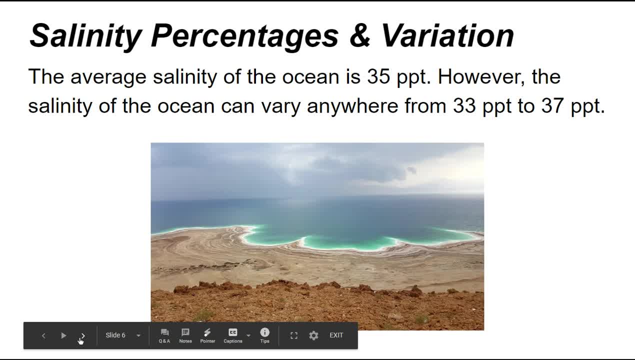 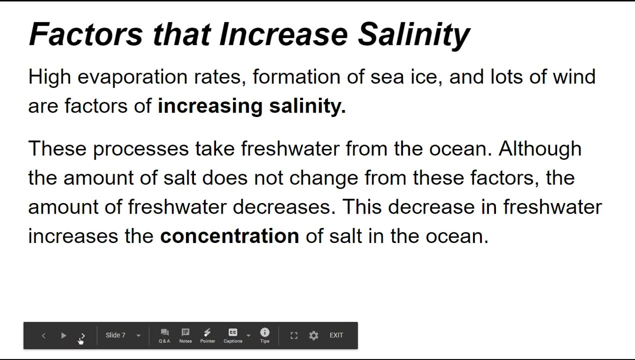 Salinity percentages and variation. The average salinity of the ocean is 35 ppt. However, the salinity of the ocean can vary anywhere from 33 ppt to 37 ppt. There are several factors that can increase salinity: High evaporation rates, formation of sea. 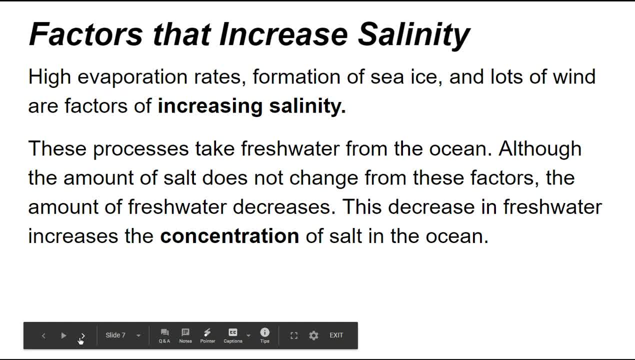 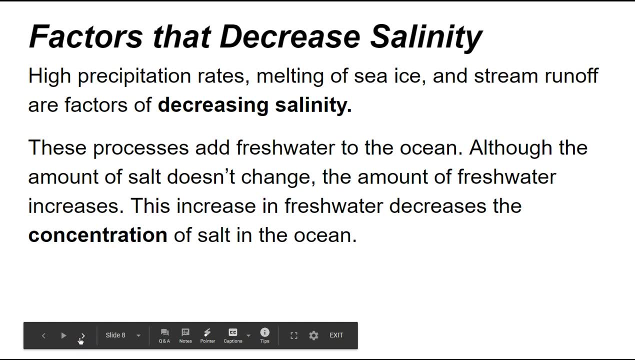 ice and lots of wind are factors of increasing salinity. These processes take fresh water from the ocean. Although the amount of salt does not change from these factors, amount of freshwater decreases. This decrease in freshwater increases the concentration of salt in the ocean. Factors that decrease salinity: High precipitation rates, melting of sea ice and 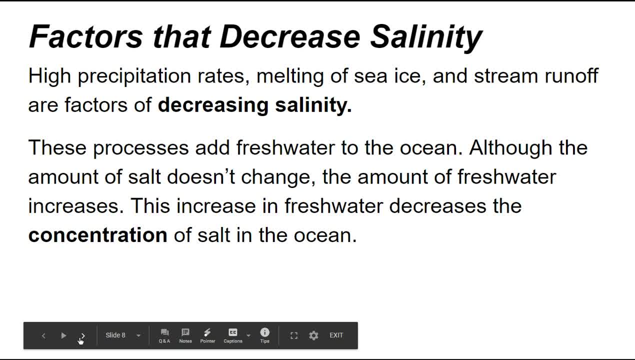 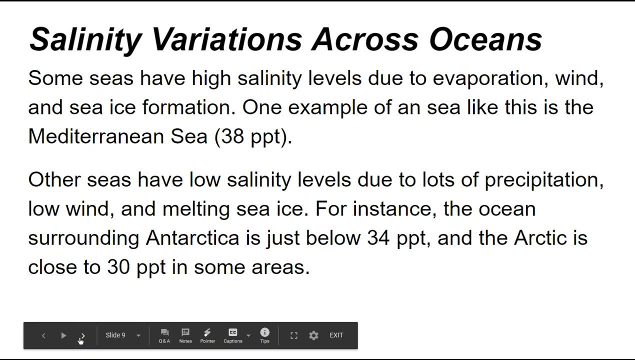 stream runoff are factors of decreasing salinity. These processes add freshwater to the ocean. Although the amount of salt doesn't change, the amount of freshwater increases. This increase in freshwater decreases the concentration of salt in the ocean. Salinity variations across different oceans. Some seas have high salinity levels due to evaporation, wind and sea ice formation. 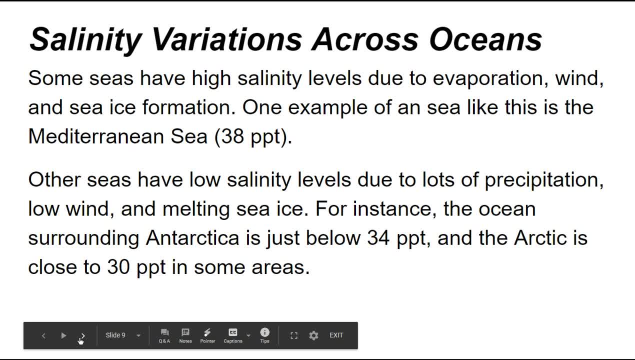 One example of a sea like this is the Mediterranean Sea. Other seas have low salinity levels due to lots of precipitation, low wind and melting sea ice. For instance, the ocean surrounding Antarctica is just below 34 ppt and the Arctic is close to 30 ppt in some areas. 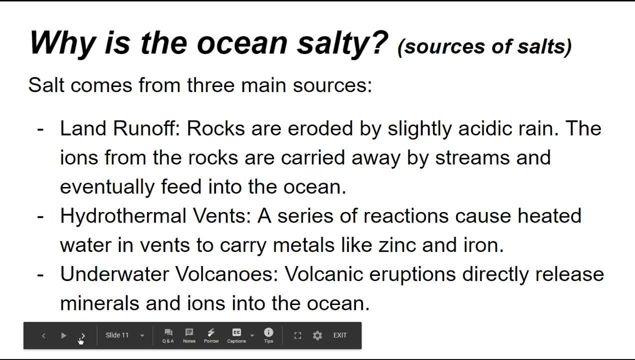 So why is the ocean salty? Salt comes from three main sources: Land runoff. Rocks are eroded by slightly acidic rain. The ions from the rocks are carried away by streams and eventually feed into the ocean. Hydrothermal vents- A series of reactions- cause heated water and vents to carry metals like zinc and iron Underwater volcanoes. 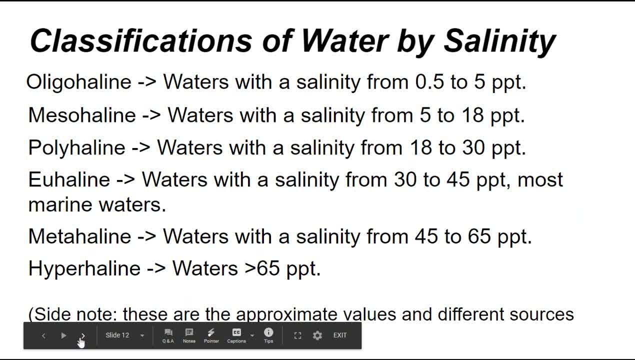 Volcanic eruptions directly release minerals and ions into the ocean. So here are the classifications of water by salinity. Oligohaline is waters with a salinity between 0.5 and 0.5.. Oligohaline is a water with a salinity between 0.5 and 0.5.. Oligohaline is a water 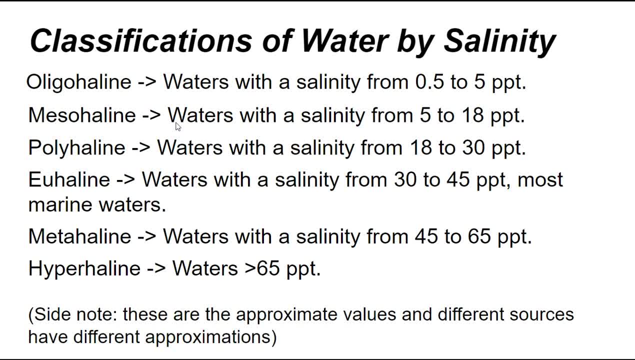 with a salinity between 0.5 and 0.5 ppt. Mazohaline is waters with a salinity from 5 to 18 ppt, Polyhaline waters with a salinity from 18 to 30 ppt, and so on and so forth. 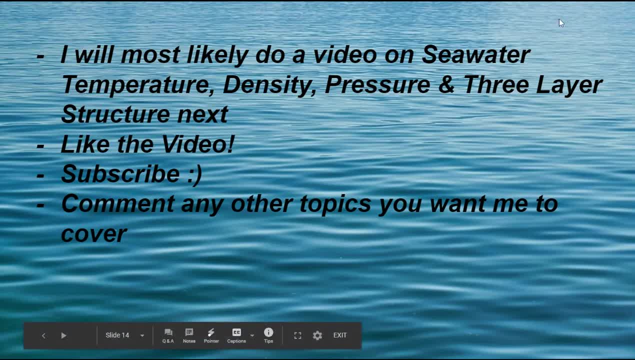 Okay, guys. this is the end of the video. Hopefully I'll make a longer one next time. Bye.